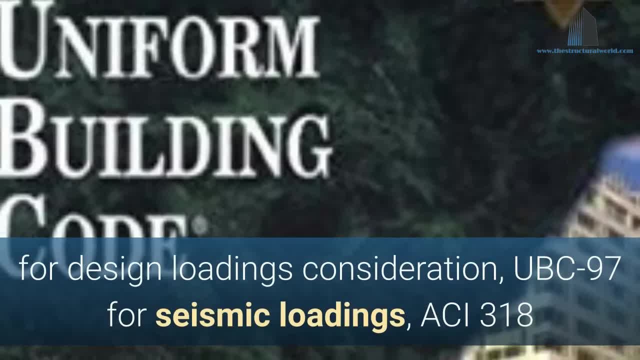 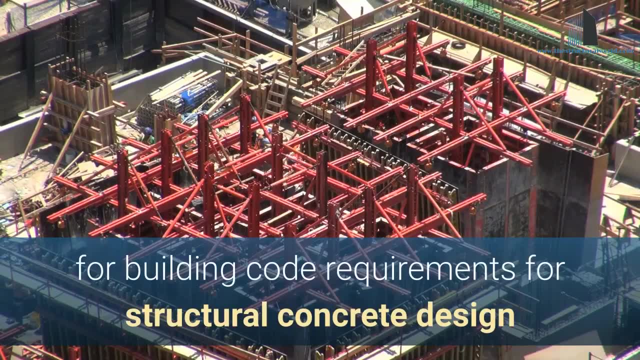 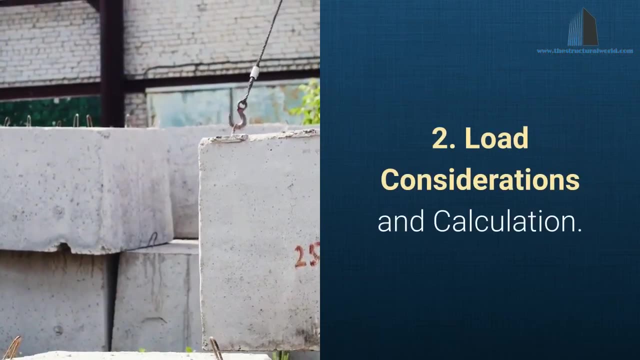 American codes, we can refer to ASCE 7 for design loadings consideration, UBC 97 for seismic loadings, ACI 318 for building code requirements for structural concrete design and AISC for steel structures. 2. Load considerations and calculation. After identifying the codes that we are going to 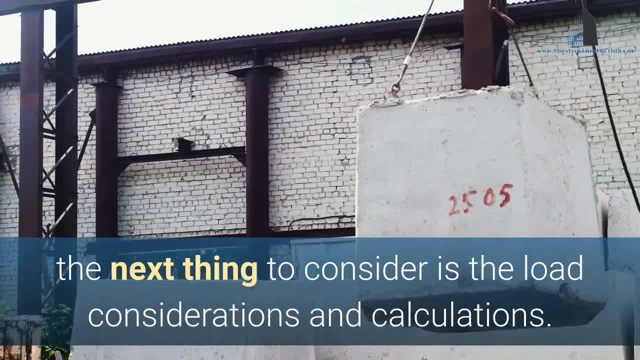 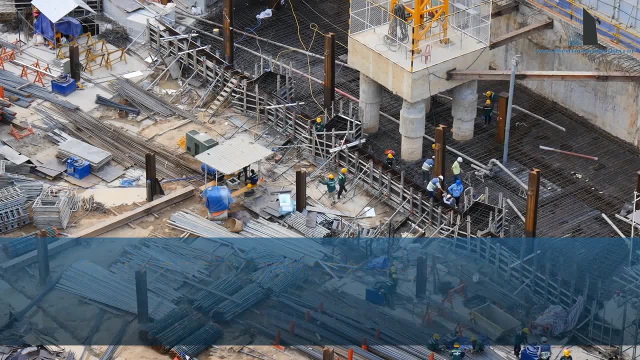 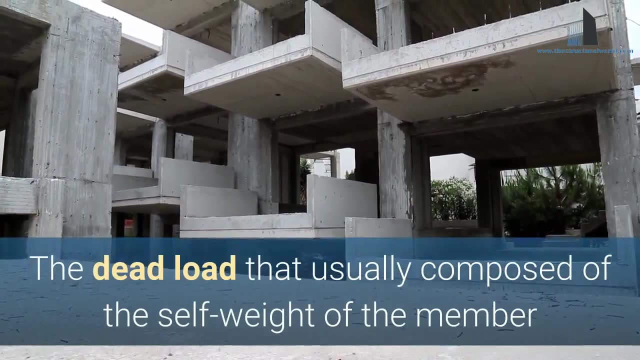 use in the design. the next thing to consider is the load considerations and calculations. The load considerations are depending on the type of occupancy of the project. Here the three basic loadings of a building are being assigned: The dead load that, usually composed of the self-weight of the member or a structure. the superimposed dead load that. 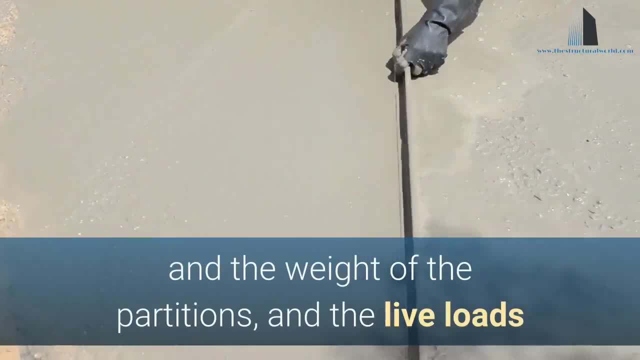 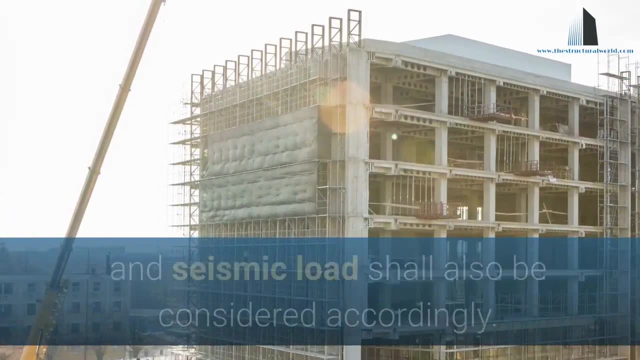 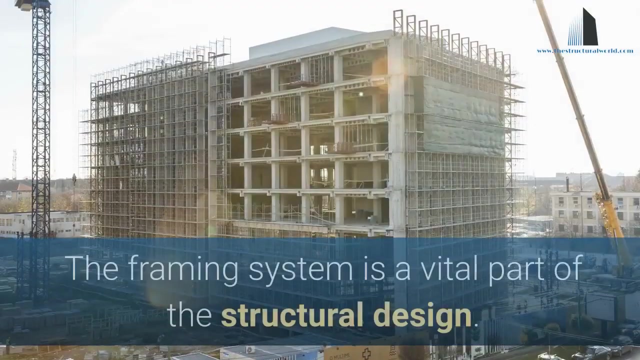 comprises of the floor finishes and the weight of the partitions and the live loads that constitute the movable loads that the structure may carry, Depending on how high the project is. a wind load and a seismic load should also be considered accordingly. 3. Propose a Framing System. The framing system is a vital 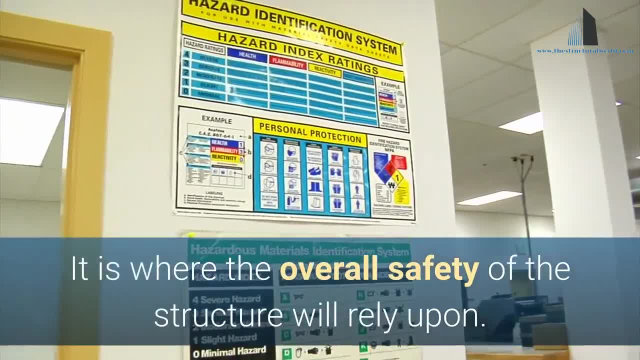 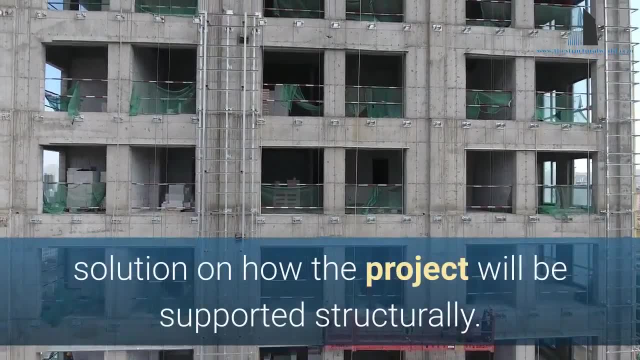 part of the structural design. It is where the overall safety of the structure will rely upon. In this aspect, the structural engineer should come up for a better solution on how the project will be supported structurally. At this stage, the designer should study and review the possible. framework of the project without compromising the safety, and soundly like a devotee should do so. gutter network androve. at the end of the construction process, Elaborately thinking about what components the project will be installed in what kind ofdad2000with this aspect, the structural engineer should come. 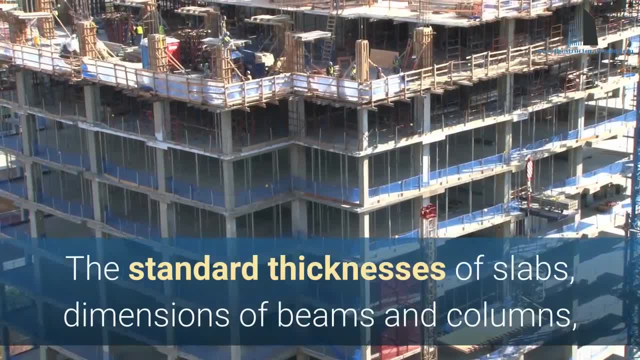 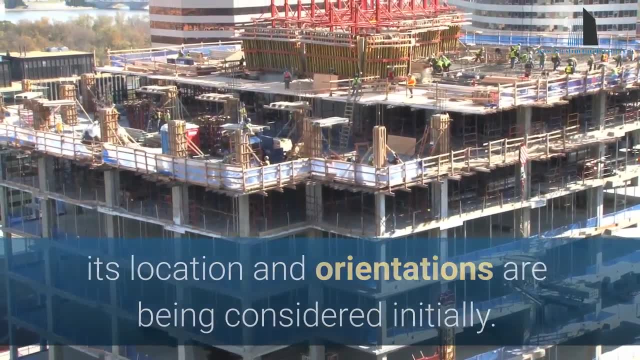 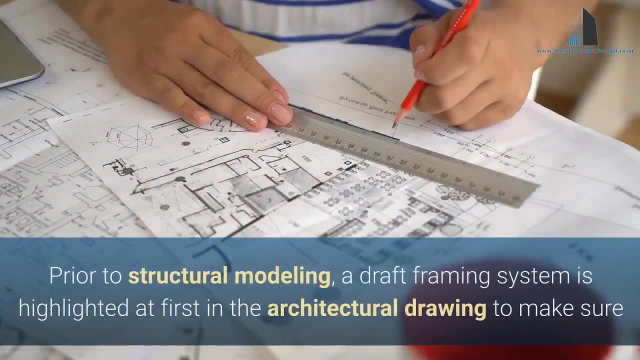 and soundly of the building that we are designing. The standard thicknesses of slabs, dimensions of beams and columns, its location and orientations are being considered initially. Proper coordination in other departments, like the architectural and MEP, should also be observed Prior to structural modeling. a 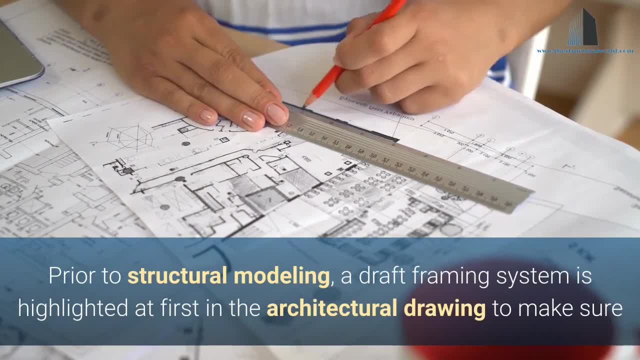 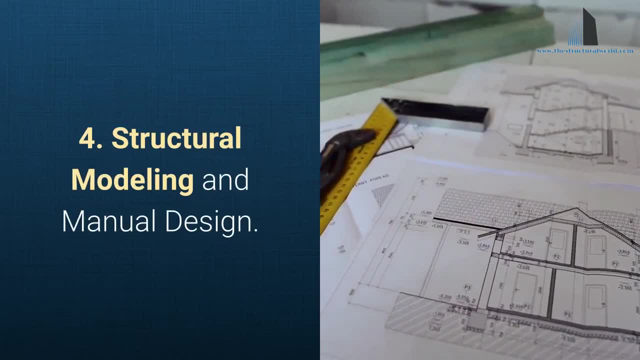 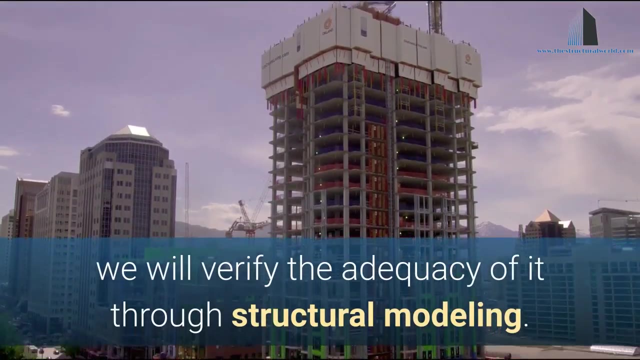 draft framing the system is highlighted at first in the architectural drawing to make sure that no architectural aspects are being compromised. 4. Structural Modeling and Manual Design. Once the proposed framing has been finalized, we will verify the adequacy of it through structural modeling, Using available 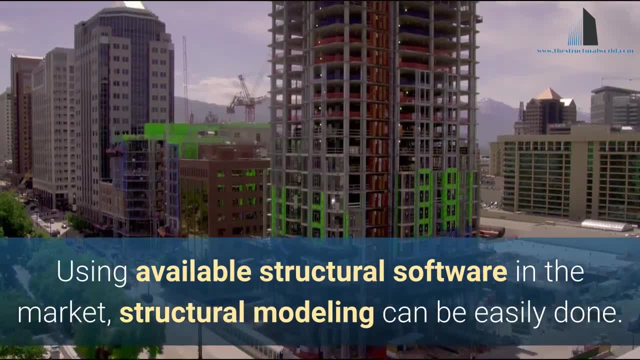 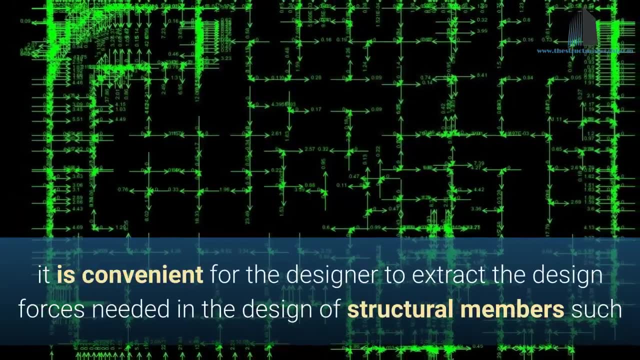 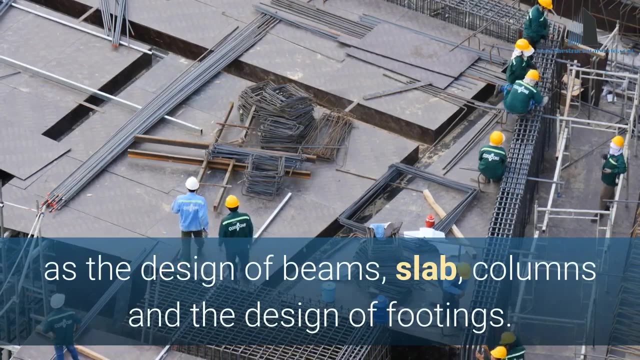 structural software in the market. structural modeling can be easily done Using three-dimensional modeling structural software like ETABS and STOD PRO. it is convenient for the designer to extract the design forces needed in the design of structural members, such as the design of beams, slab columns and the